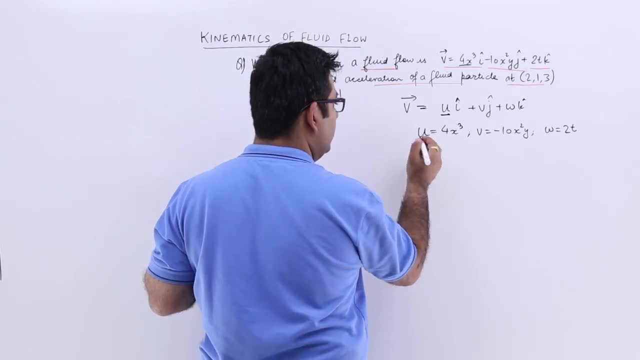 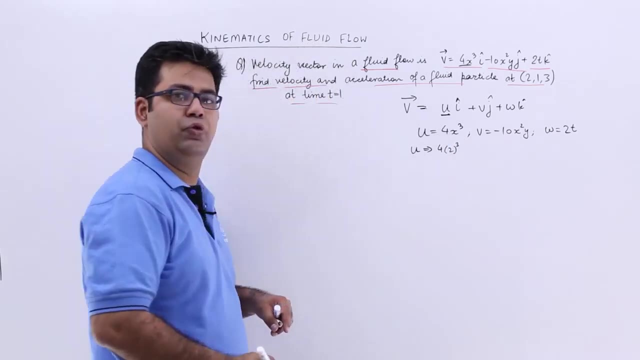 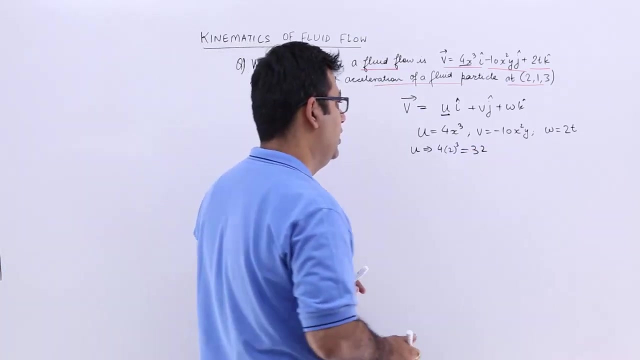 point u will be equal to 4x2 cube. Okay, so this will be 8x4, 32.. Now I don't know what units are we using- meters per second or fourths per inches? So let's write it down just 32. 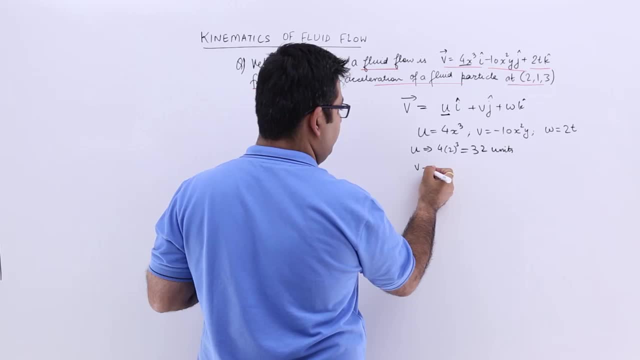 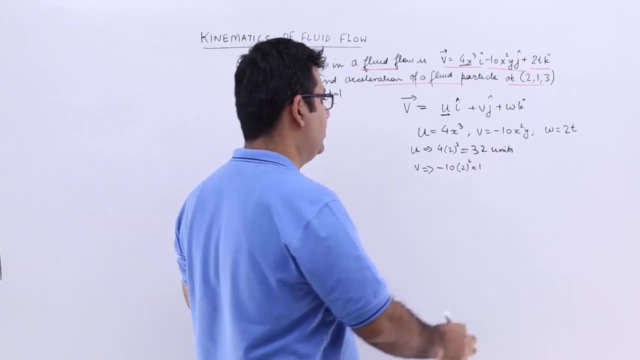 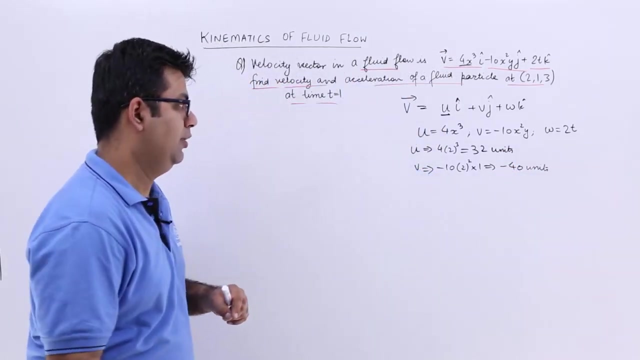 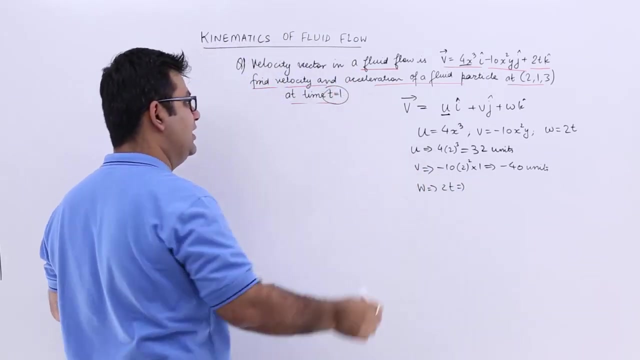 units simply. Then we write down v. v would be minus 10, 2 square into 1.. So you get minus 40 units. Then w is equal to 2t, T is equal to 1. So it will be equal to 2 units. So I can put. 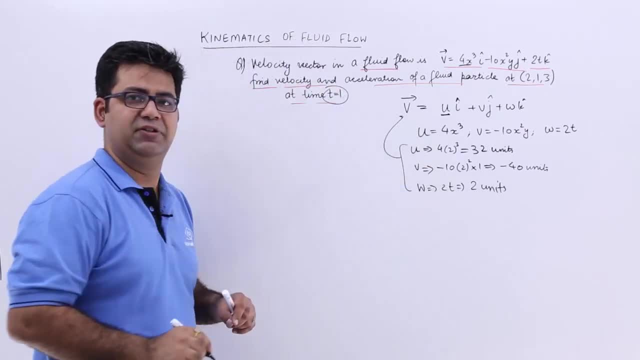 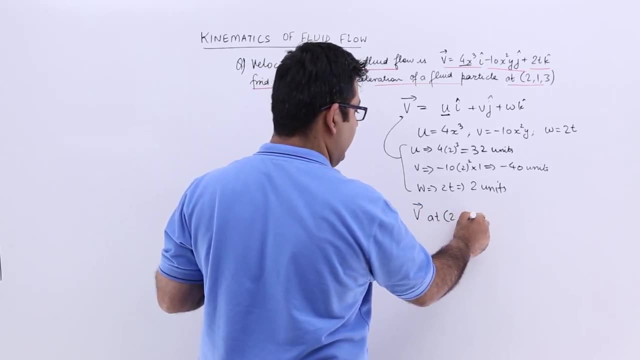 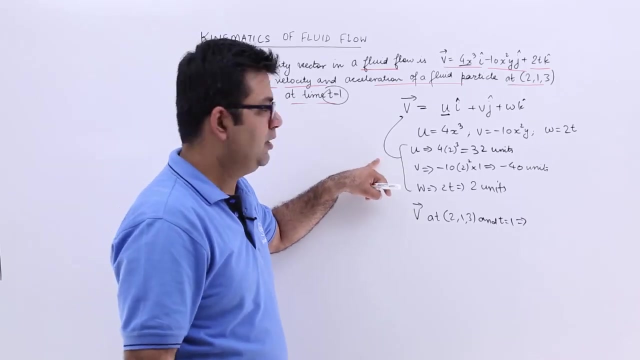 the value of uv and w into this velocity function. So you will have velocity vector v at point 213.. Okay, and t is equal to 1. this can be written as 32 i cap minus 40 j cap plus 2 k cap, so you: 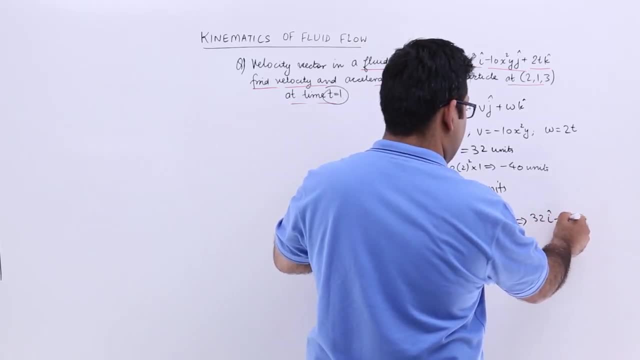 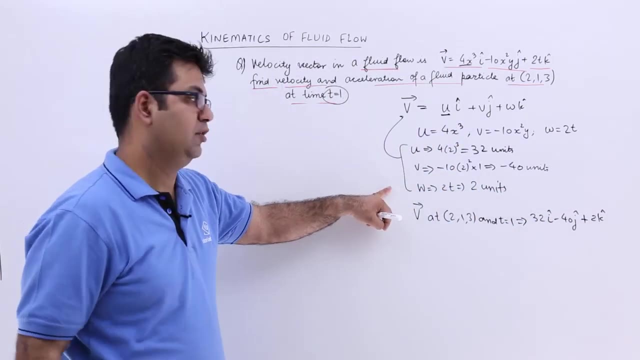 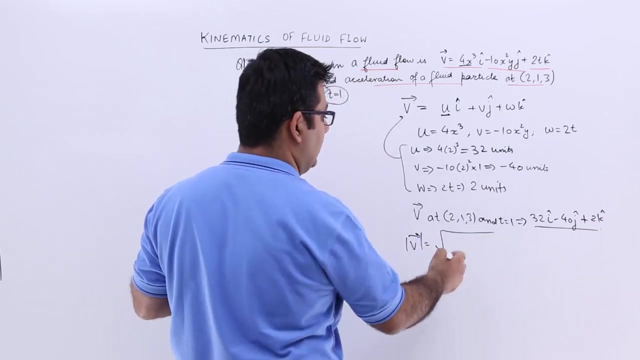 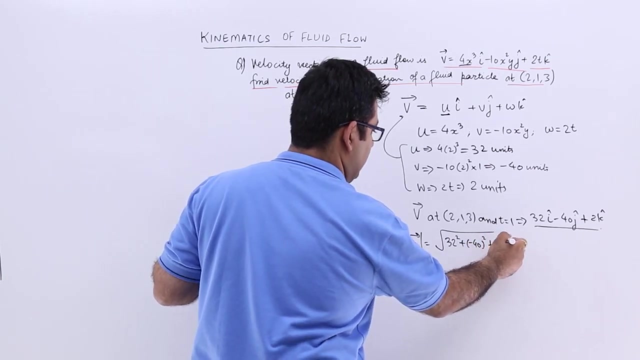 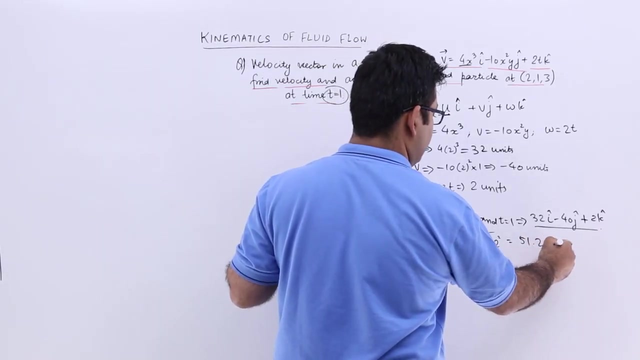 will have 32 i cap minus 40 j cap plus 2 k cap. so this is the velocity vector. to find out the magnitude, you will have to simply find the mod 32 square plus minus 40 square plus 2 square. so this would give you a value which is equal to 51.26 units. so the velocity 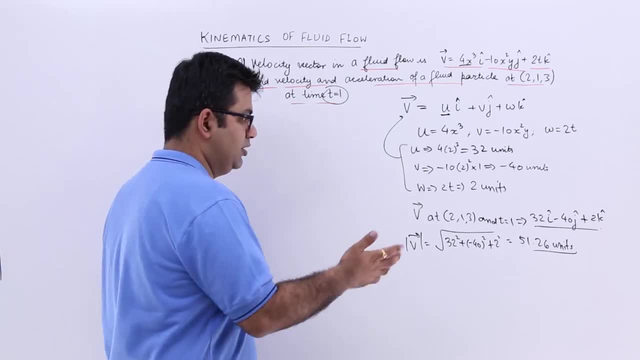 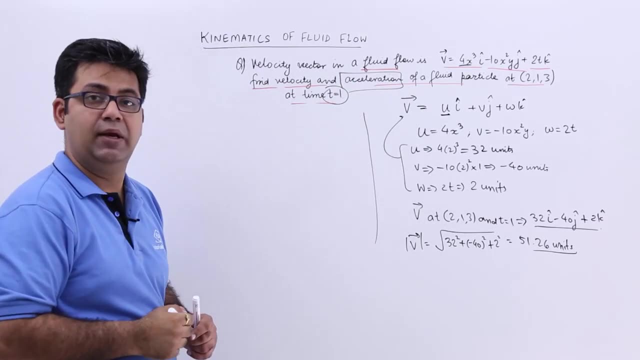 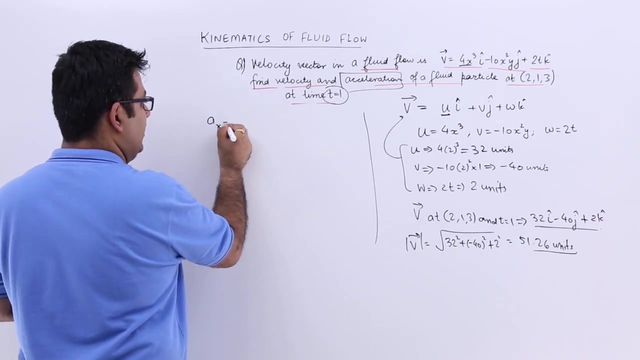 is 51.26. units may be meters per second, or centimeters per second as well. alright, so this is the velocity. now we have to find out the acceleration as well. there are 3 components: ax, ay and az. so ax, what was a x equal to, it was u into curly u by curly x plus v into curly u by. 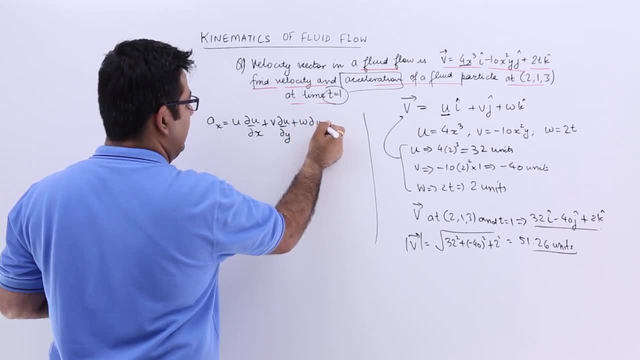 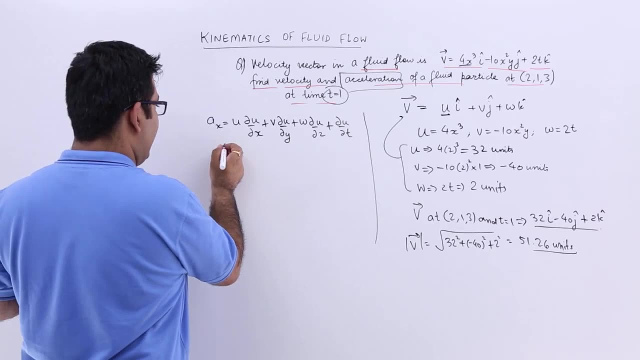 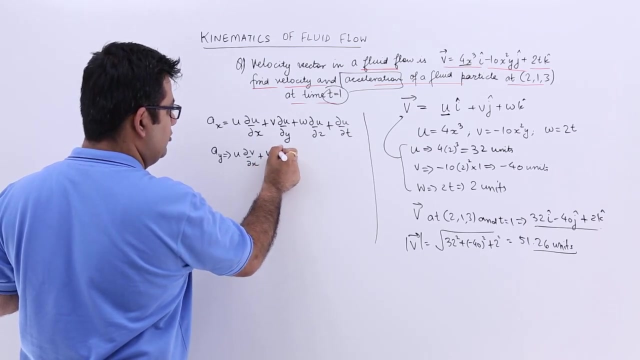 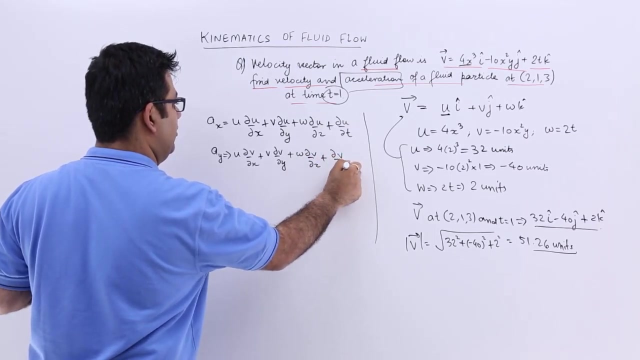 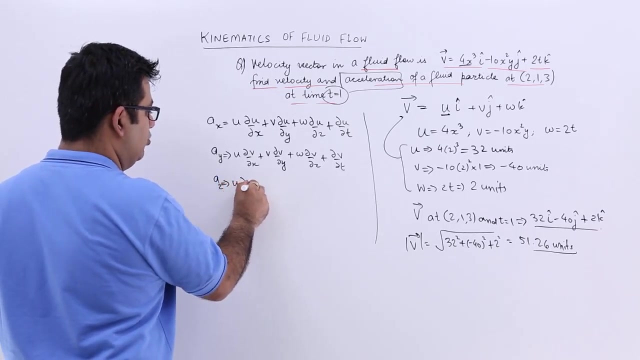 curly y plus w into curly u by curly z plus curly u upon curly t. similarly i will have ay, this will be u into why curly v upon curly x plus v, into curly v upon curly y plus w into curly v upon curly z plus curly v upon curly t, and then az it would be u into curly w. this is not yeah- by x plus. 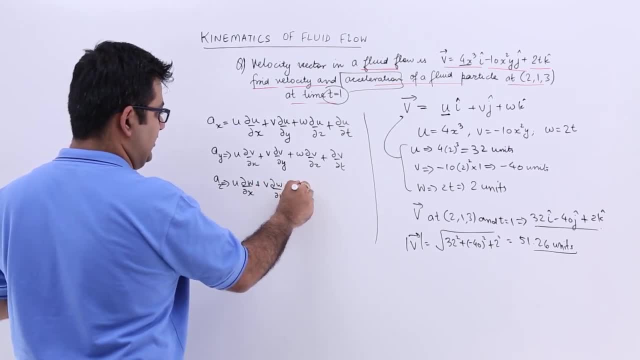 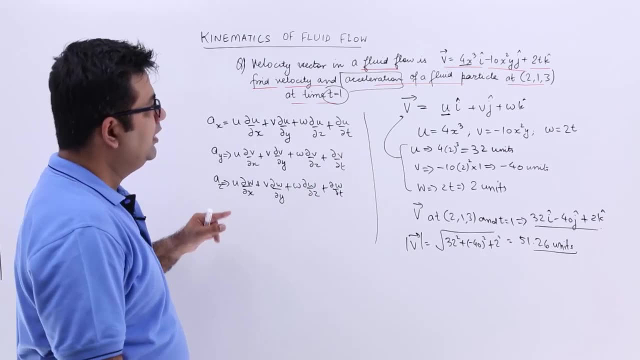 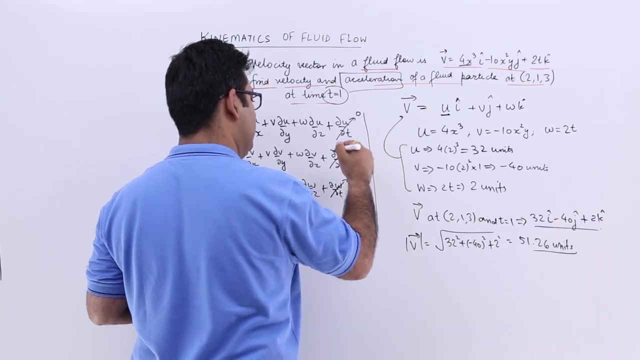 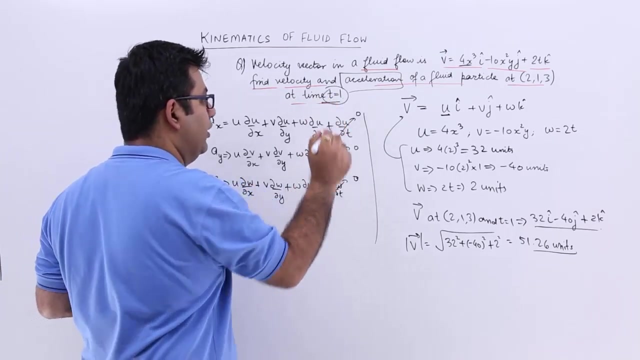 v into curly w by curly y plus w into curly w by curly z, plus curly w by curly t. now let's assume the entire flow is steady flow, so all these values would become zero. so all these values would become zero. okay, but no, you have a time value given to you. this means your. 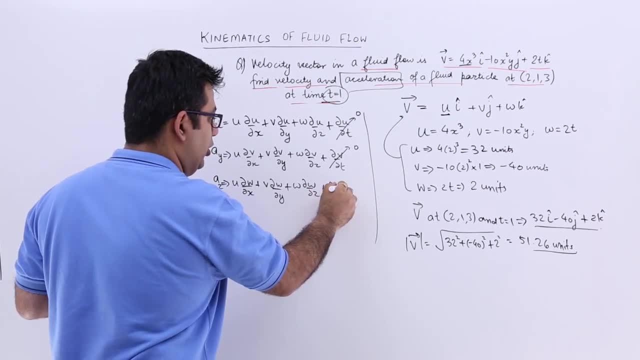 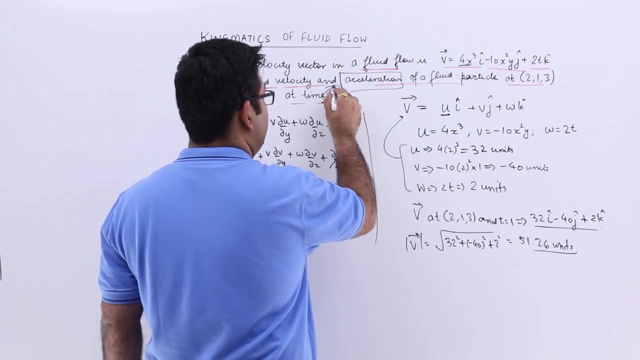 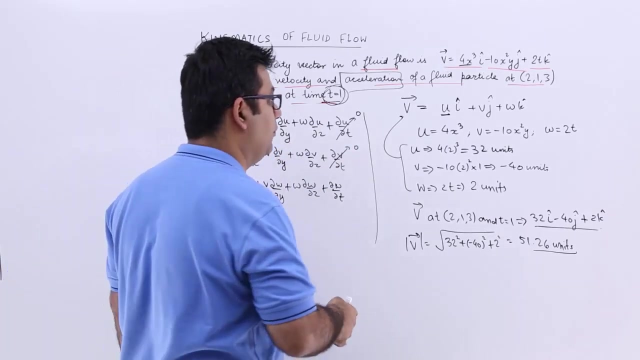 curly w by curly t, It is not going to become zero. so you have some variation of velocity in the graduate z direction. so this is something we need to, you know. just check before just blindly striking off the w component also, so you can see u is only a function of x and y. let us say v. 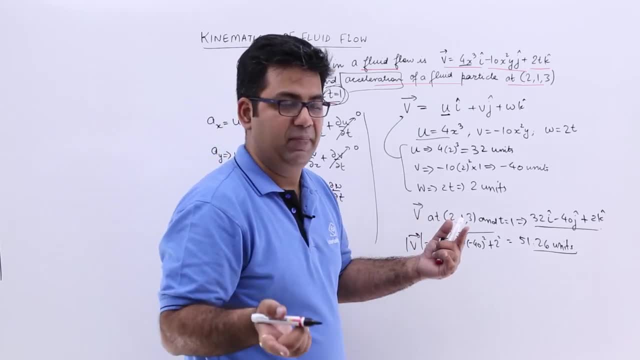 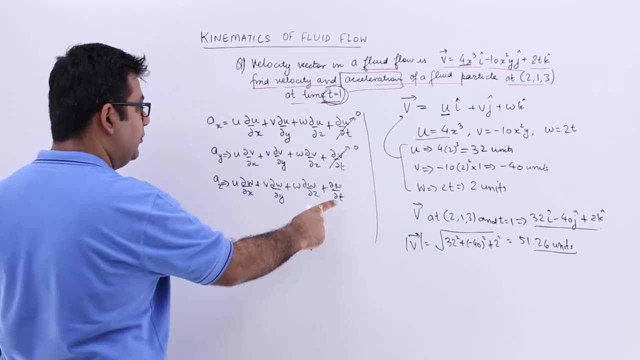 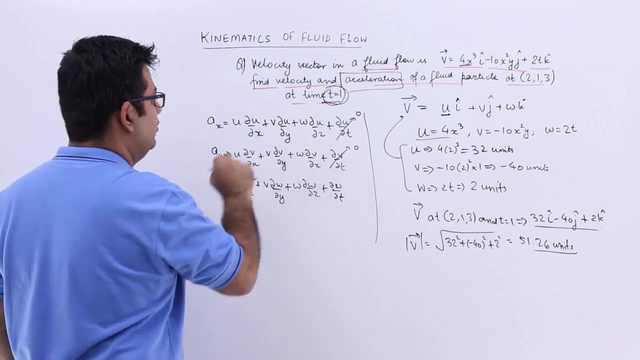 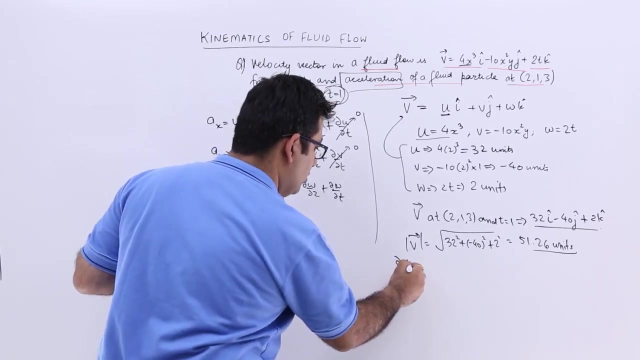 is also a function of only x and y, but w is a function of time, so w will not become so on to this term will not become 0. ok, so we can easily find out these values. so if you look at this, curly u by curly x, you can find it from here. so you will have curly u upon curly x. this is. 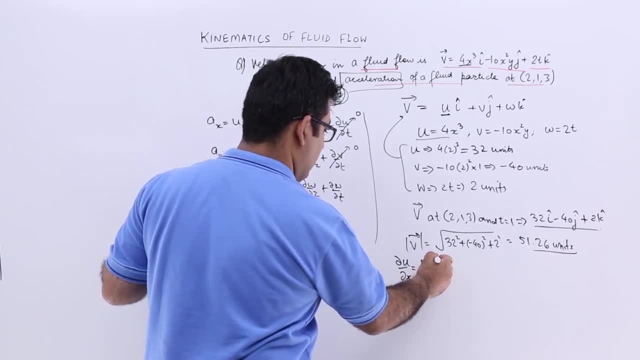 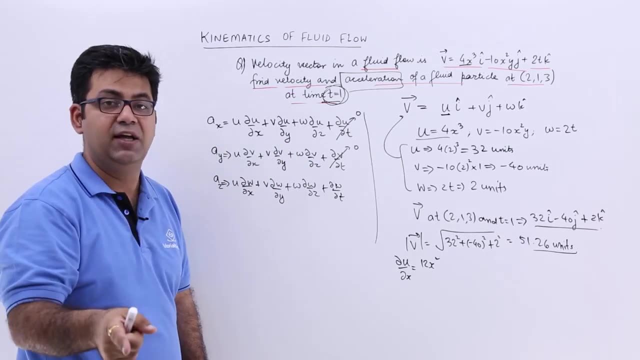 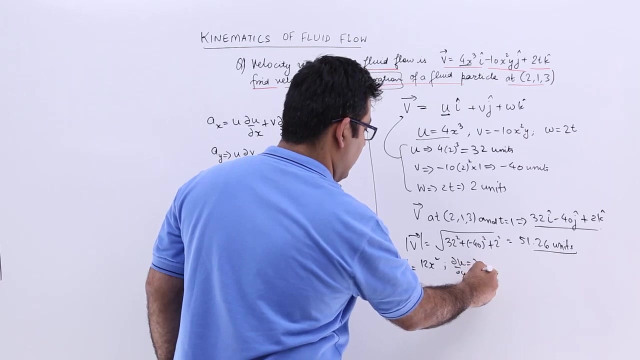 12 x square. ok, and all these two values, that is, the differentiation of u with respect to y and z, would be 0. so I can straight away write down: curly u upon curly y is equal to curly u upon curly z, which is 0. ok, and the variation of u with respect to t is already. 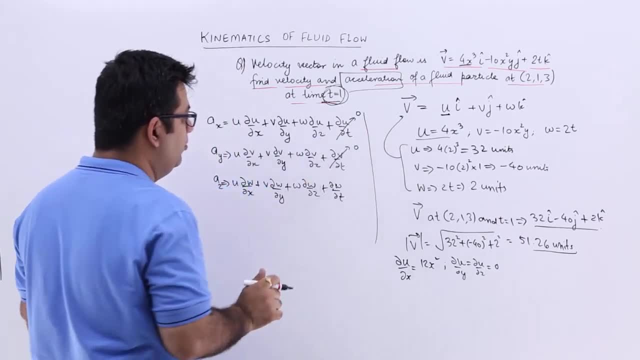 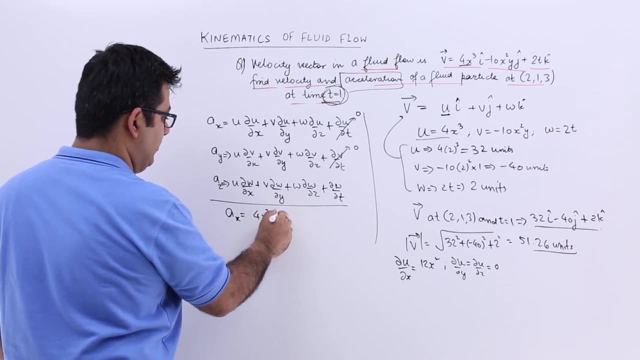 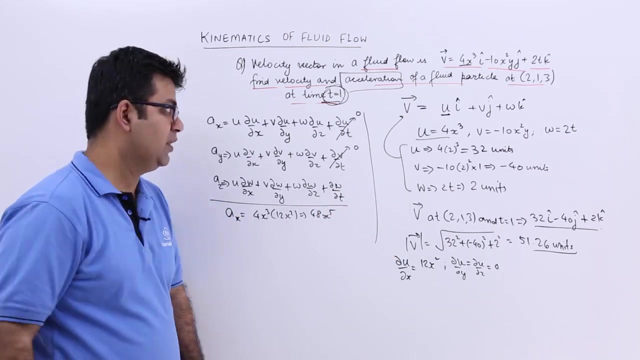 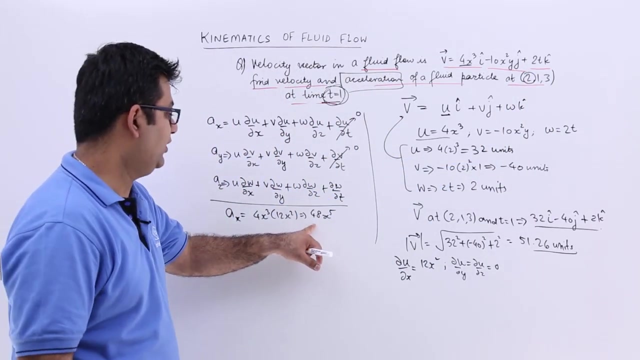 0, so u is given to us as 4 x cube. so I can write down ax as 4 x cube into 12 x square, which is 48.. x to the power 5. now I can simply put x as 2 over here, ok, so you will have 48 into 2. 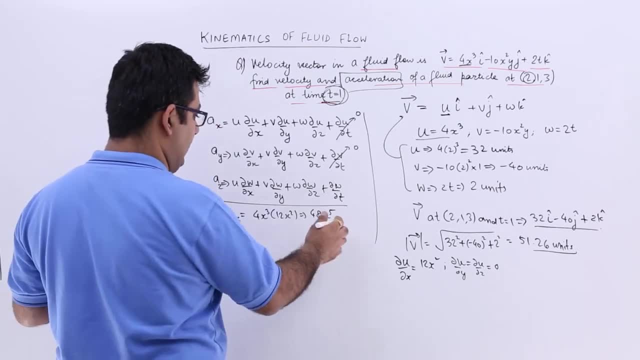 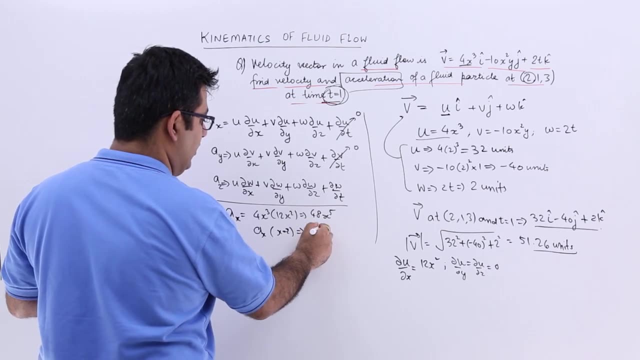 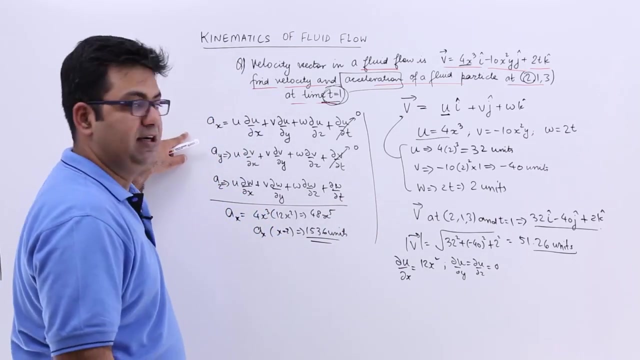 to the power 5 right, and that would give you a value of ax at x is equal to 2 as 1536 units. so you have the acceleration in the x direction. Now you can easily find out what is the acceleration in the x direction. 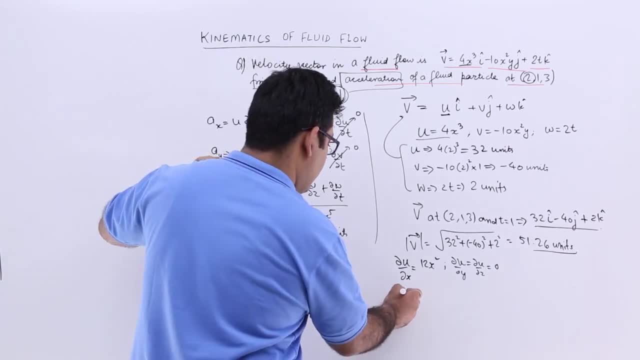 Now you can easily find out what is the acceleration in the x direction. So you can easily find out what is the acceleration in the x direction. So you can easily find out what is the acceleration in the x direction, Notice, by calculating curl e x again. so curl e x to the power 4 will be equal to curl v. 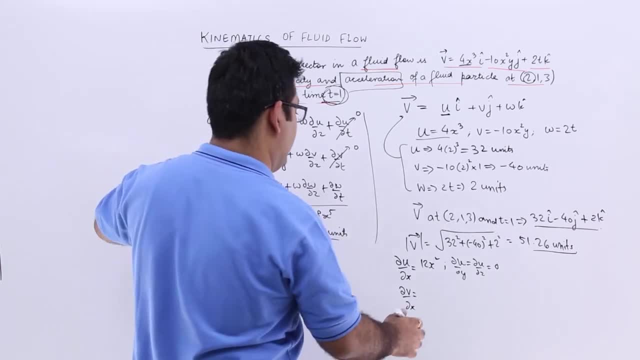 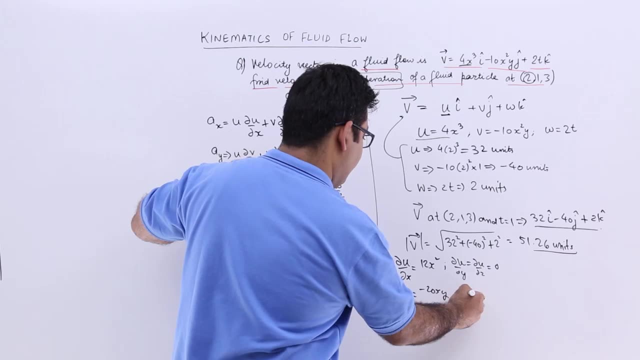 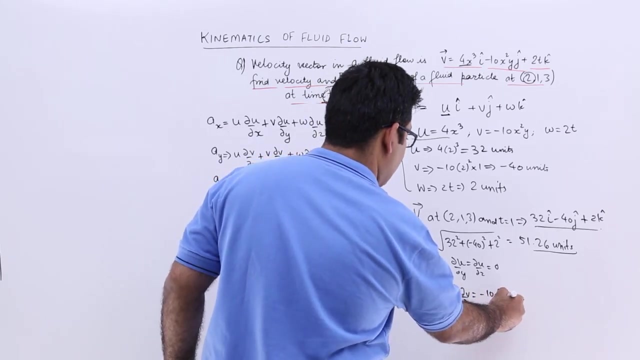 upon curl x, so curl e x will be x, which is 10 time. Lewis f circle щ into Your our curl V left hand declaration. So this is a curly v called curl V by curly x. so curl V upon curl v would be how much. 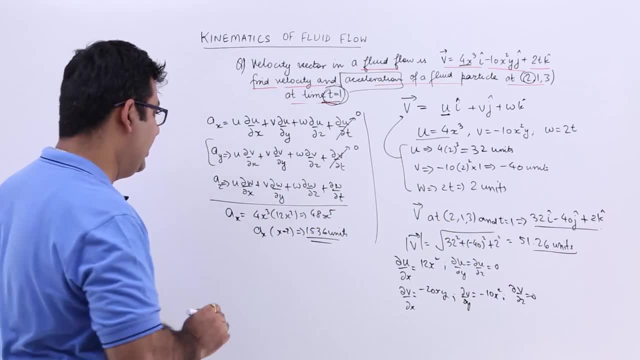 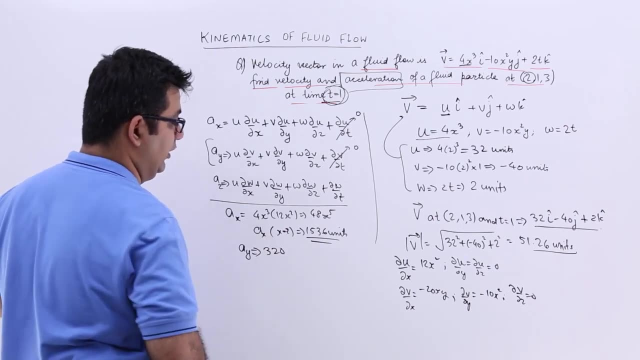 you have minus 20 xy. ok, and then curl v by curl V would be how much? curl v upon curl V would be minus 10 X square, minus 10 X square. and then curl v by curl Z would be 0. so from here the values in this expression and find out the value for a y that will be three twenty. 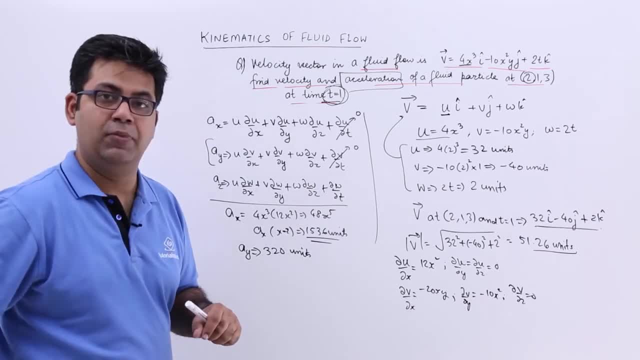 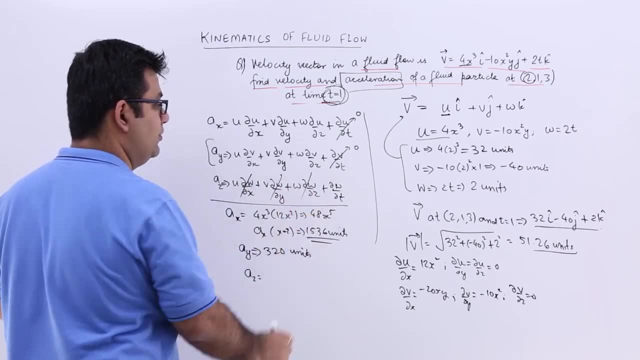 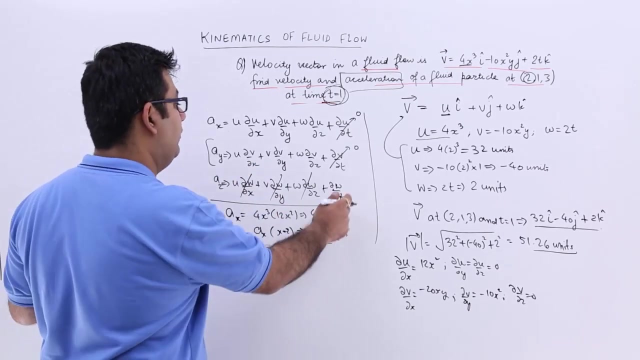 will be three, twenty units. ok. similarly, i can find out a z for a z. this would be zero, this would be zero, and this would be zero because there is no variation of w in x, y and z. you will only have variation of wt, and that is how much? two from here. this is two. 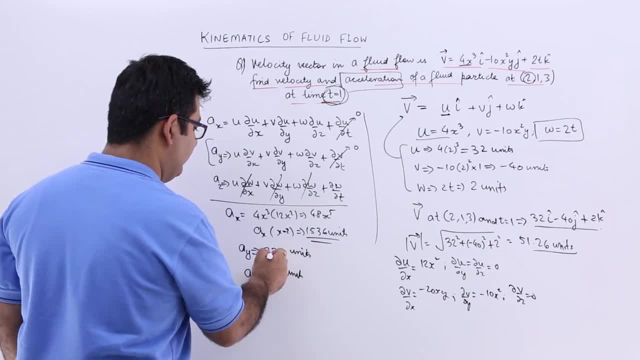 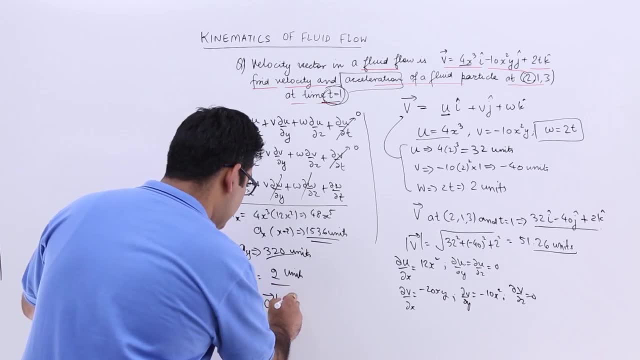 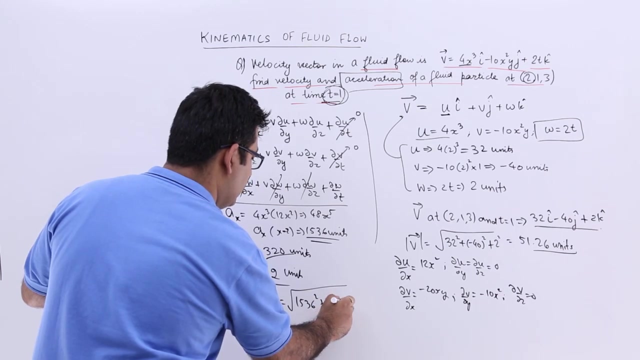 all right. so you have the three accelerations in the three directions. now the magnitude of the acceleration. a mod can be given as fifteen, thirty six square plus three, twenty square plus four, that is two square. so when you find out the value, So when you find out the value. 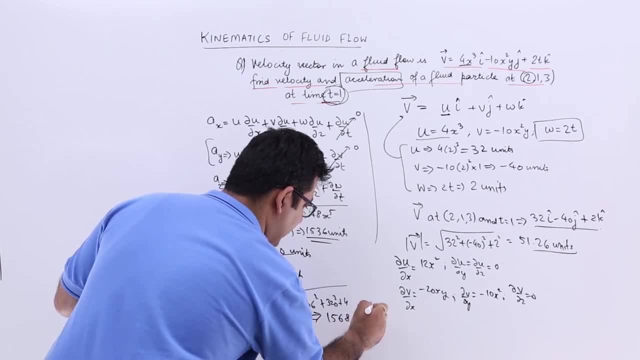 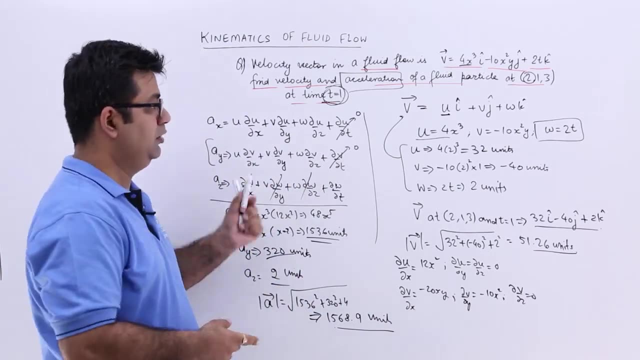 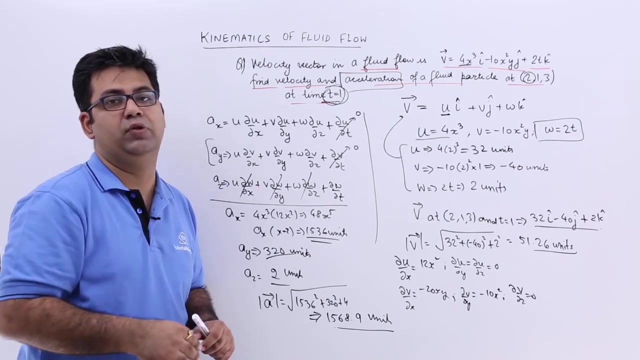 So when you find out the value, the acceleration comes out to be 1568.9 units. okay, So this is how you do a question on the topic of velocity and acceleration in fluids. Let us have a look at one more question before moving on to the next topic.